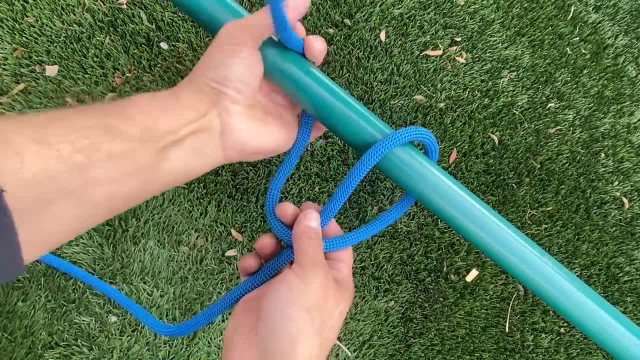 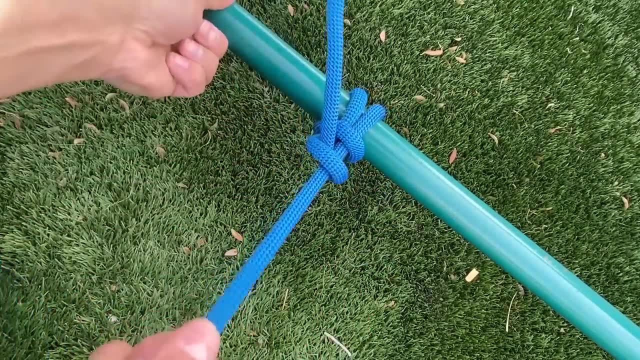 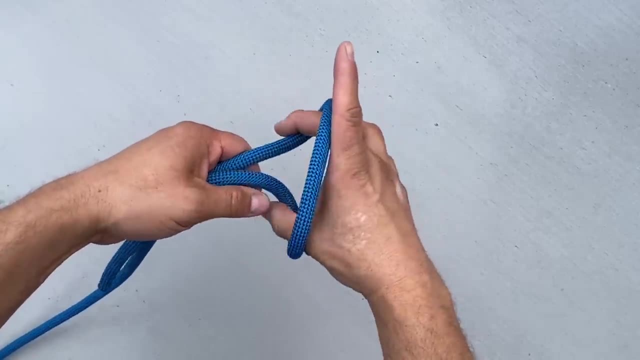 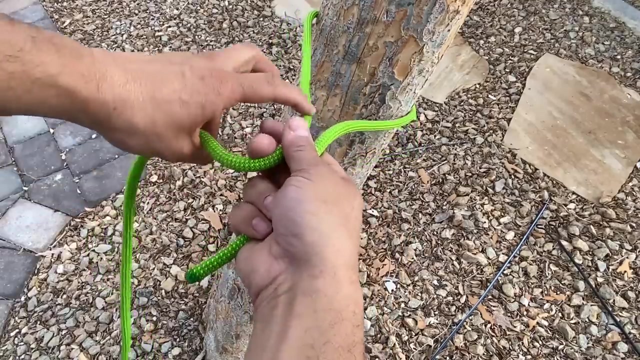 but if we were to tie this in and add a half hitch, it works well. Another way to form a cow hitch is to take a bite of our rope and put our fingers through, pinch around and together. Now, let's say I wanted to tie off to this tree, I'll form my cow hitch. 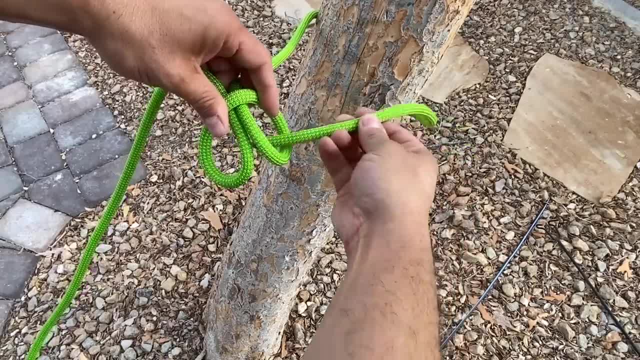 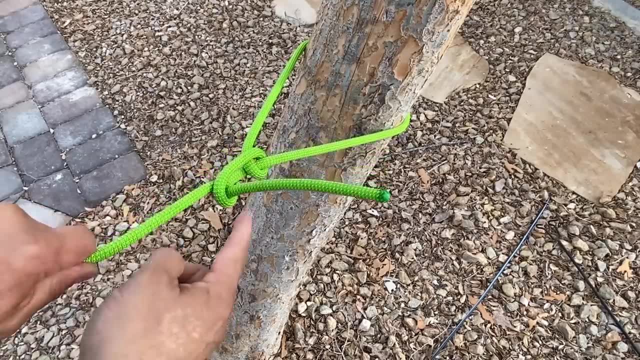 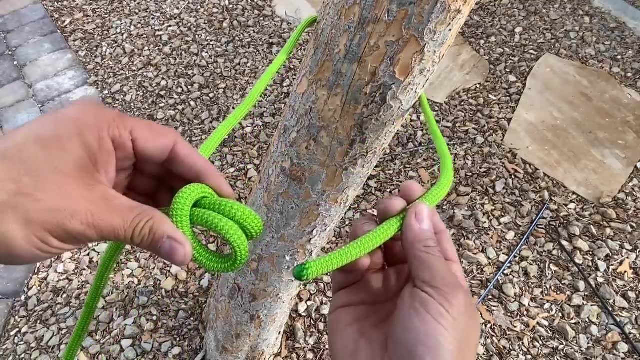 by pinching around. and now I'll just run this end right through. Let's pull this tight. Watch what happens when I pull tension on it: This end starts to slip away, and if I pull too much it's going to spill. Okay, let's try that again. I'll run my end through. 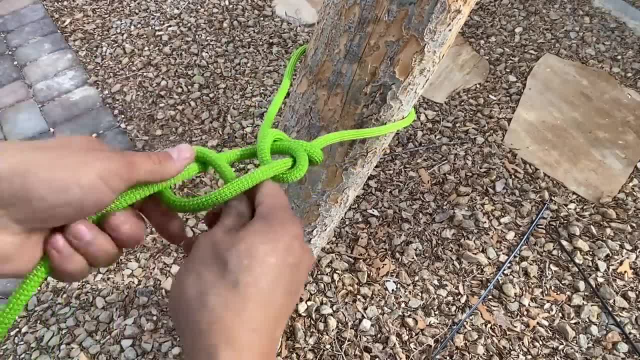 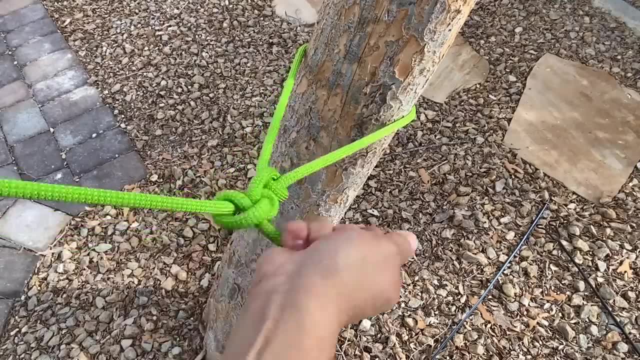 pull it tight. This time I'm going to add a half hitch on top. Now, this might work, but we can already see that this isn't cinching down enough because of the type of rope we have. So let's see what else we could do. What if, instead of doing a half hitch, 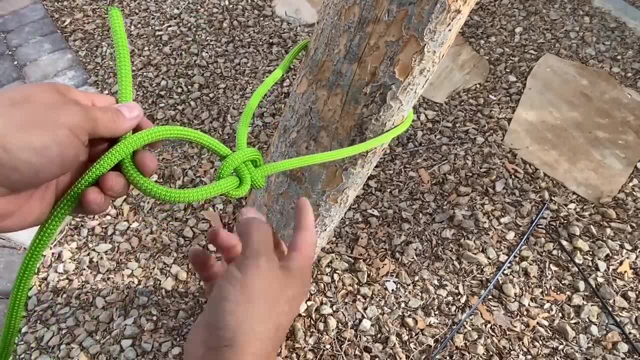 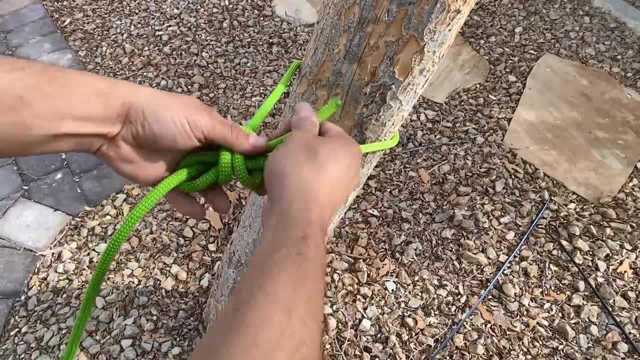 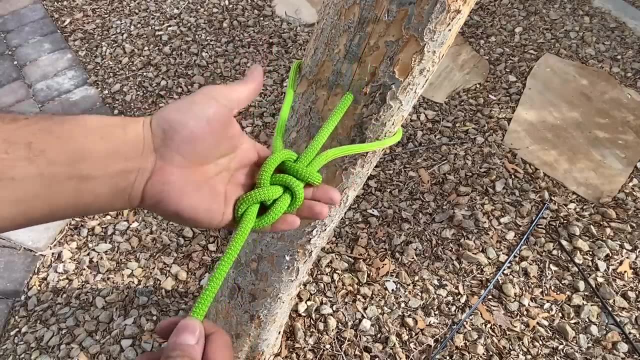 I just ran my rope around the back and right back through that cow hitch, So let's do that. Run it back through. Okay, Take a look at this. You might recognize this as a reinforced bowline. This is extremely stable. In fact, the bowline is so stable we don't need this extra turn back here. 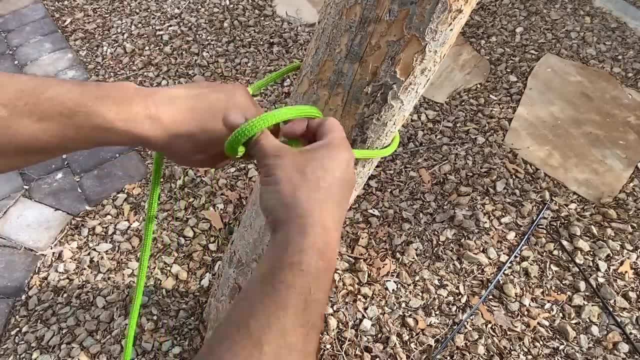 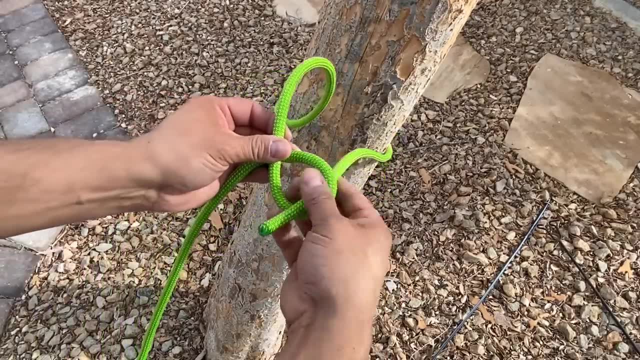 So let's tie this again. without it, I'll pull in my cow hitch on the left. Now remember, I only need half of it, so I'll let this one go. I'll run my end through, I'll go around and then back through that half hitch. I'll run my end through, I'll go around and then back. 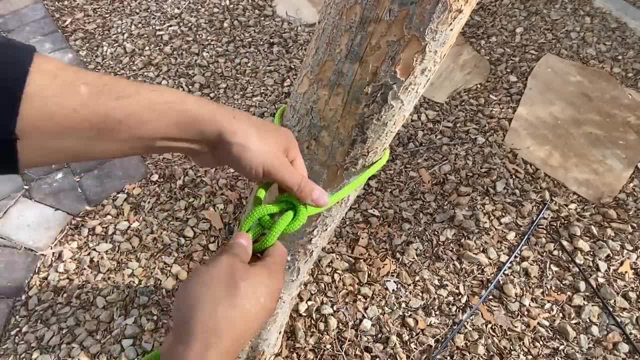 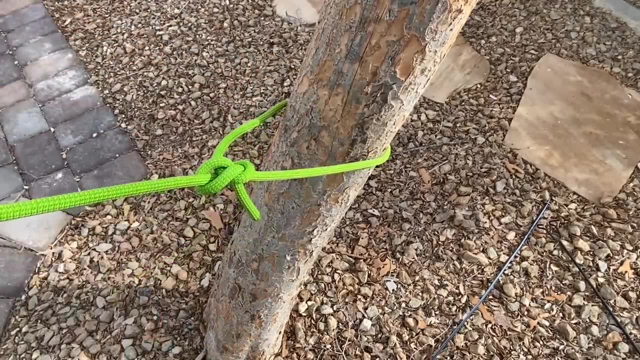 through that half hitch. I'll run my end through, I'll go around and then back through that half hitch. Let's pull this tight, All right? See, even the rooster agrees It's a good knot. All right, let's use paracord and the 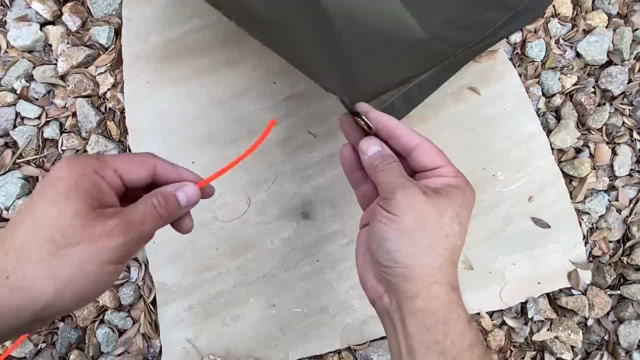 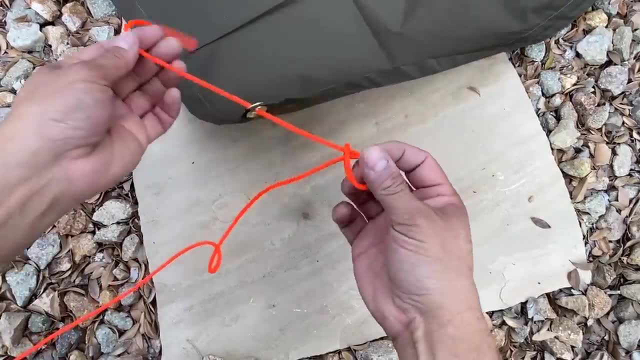 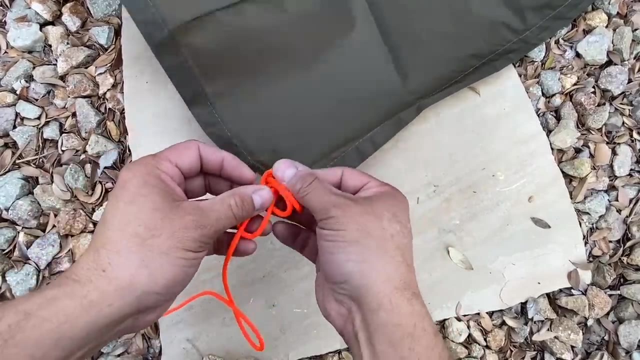 knot. we just learned to tie off the corner of this tarp. We'll run our cord through the grommet. Now I'll pinch in my cow hitch. I'll run my cord through the cow hitch around the standing portion and then back through again. 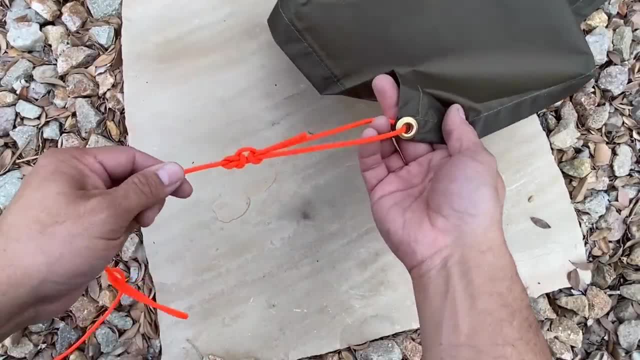 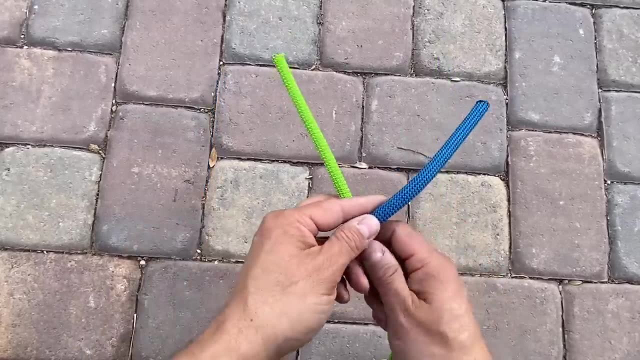 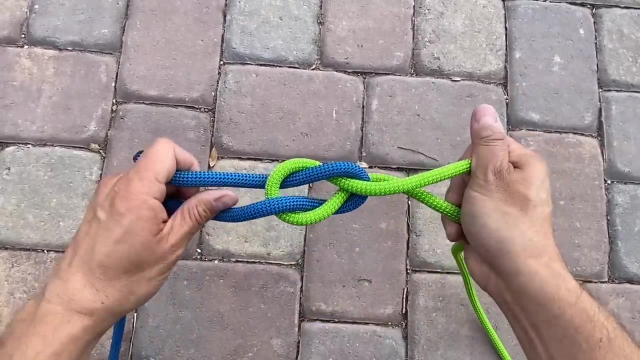 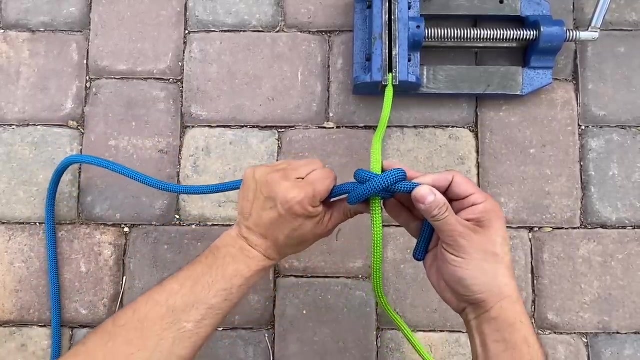 We'll pull this tight. That won't go anywhere. Now what if you tie your shoes the incorrect way using a granny knot? You go left over right, left over right. This looks similar to a square knot, but it's nowhere near as secure If we pull one in straight on our granny knot. watch what we get. This is a clove hitch. 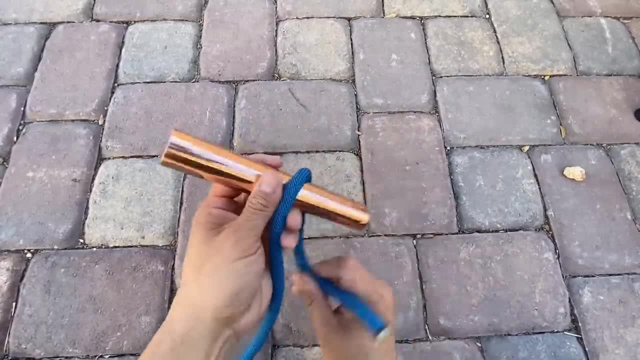 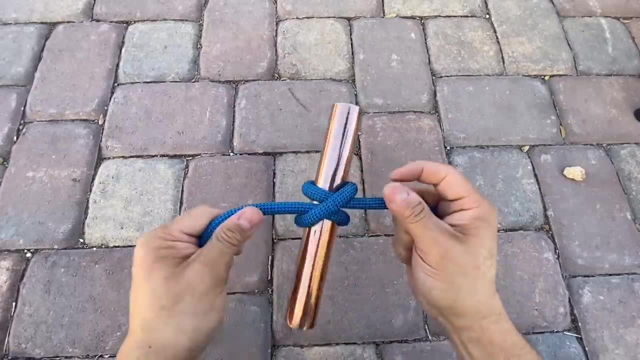 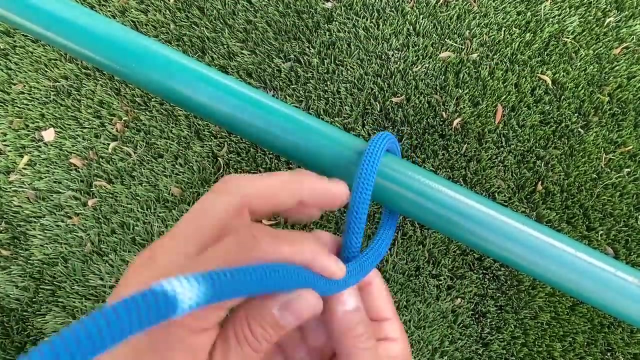 Here it is tied on the bar Left over right and wrap it around Left over right. wrap it around, Pull it tight and there is our clove hitch. We'll tie a clove hitch by going around our bar. We'll cross over the top. 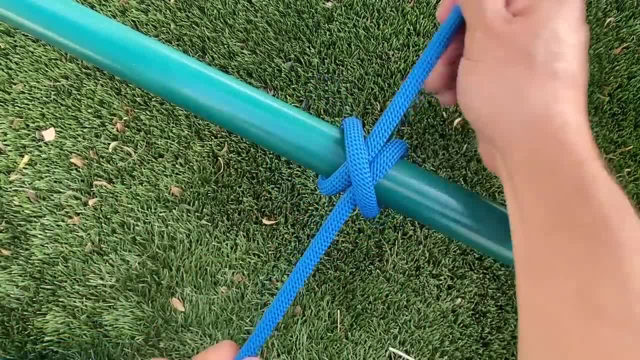 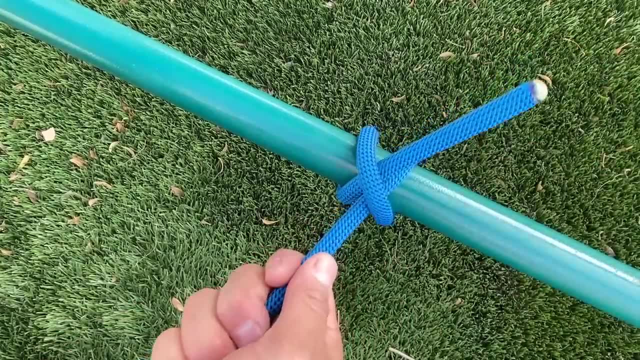 and then we'll tuck underneath that. first turn we did. This knot works best when we have tension applied equally in both directions. Tension in only one direction can cause it to slip free. This is a knot you can use for multiple anchor points. 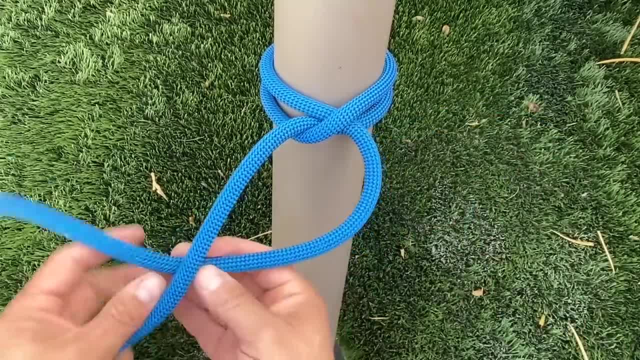 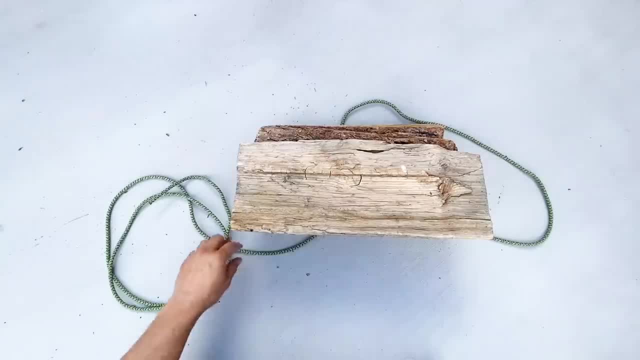 arborists use it to tie off to multiple branches. now, if you're using this to tie off to something, you always want to add a couple half hitches to make sure it stays secure. earlier we tied off to a tarp. now we are going to tie together some wood and we're 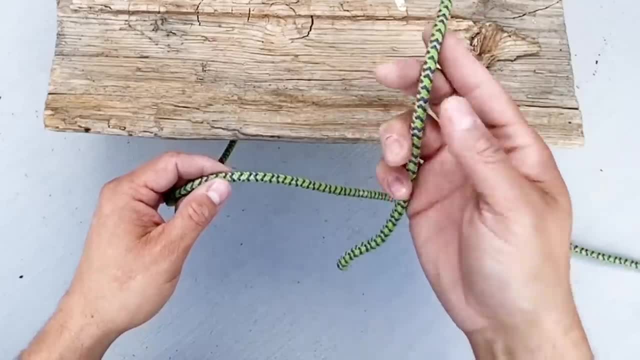 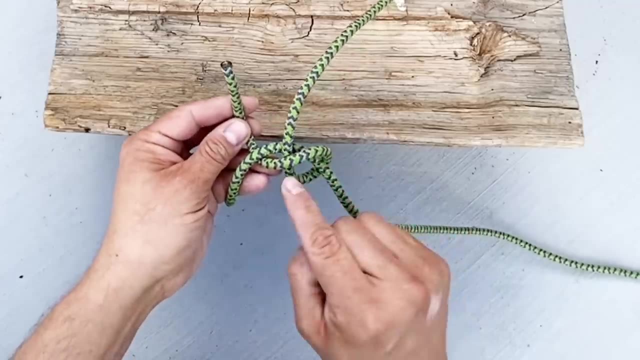 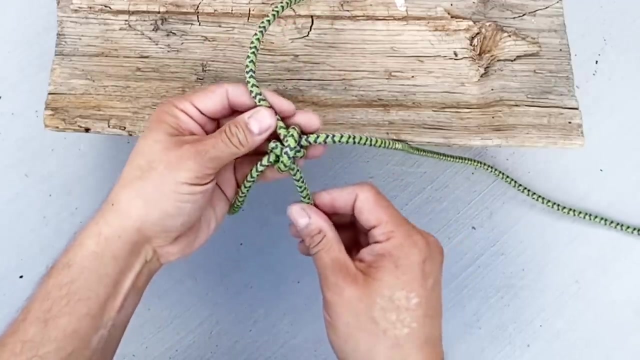 going to do that with a running clove hitch, so i'll take my rope here, i'll go over the top, go around and as i come up i'll just go back underneath that first turn that i did. there we go. now. when i finish tying this off, i'm going to use this end here. 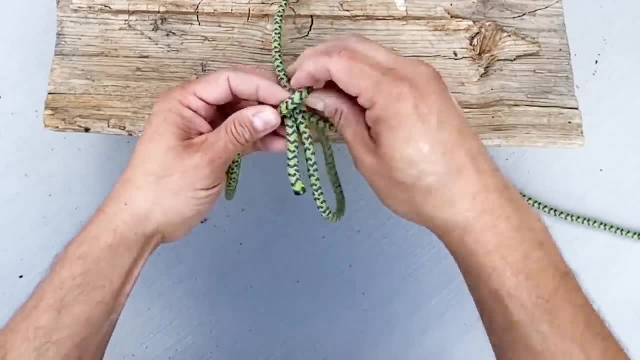 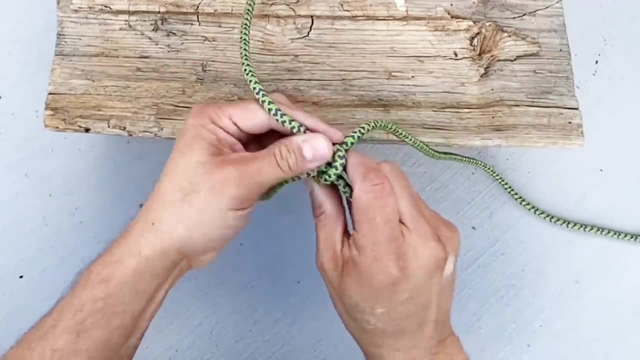 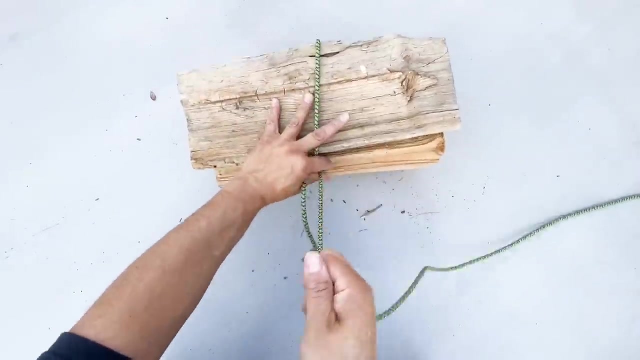 so i need to give myself a little more room. there we go now. let's just dress this up and pull it tight. our clove hitch is running up and down and we'll pull our rope through to tighten everything up. now i'll just add a couple half hitches to finish it off. 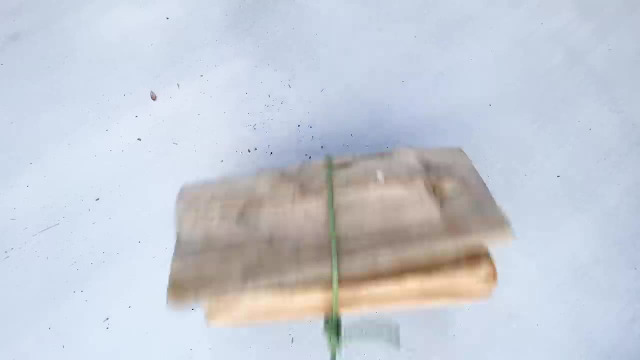 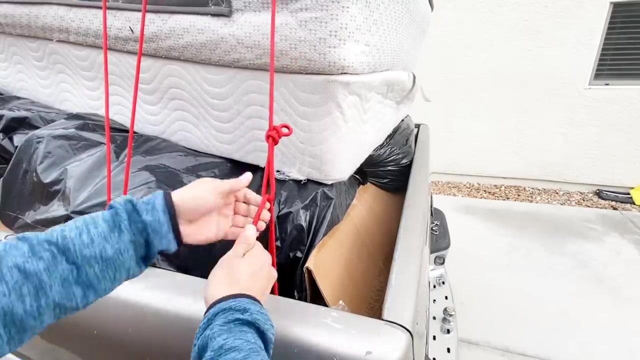 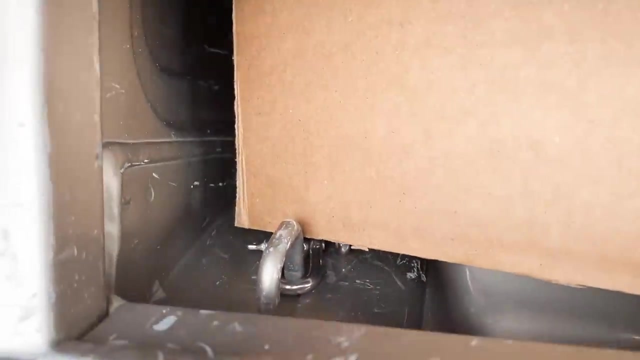 so we've tied off the corner of a tarp, we've tied together some wood and now it's time to use both knots. we've learned to tie down this strip to the dump, and we're going to start by tying off to this anchor point right down there. i've already hooked. 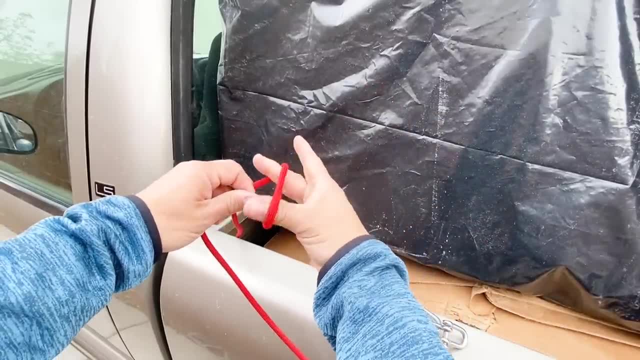 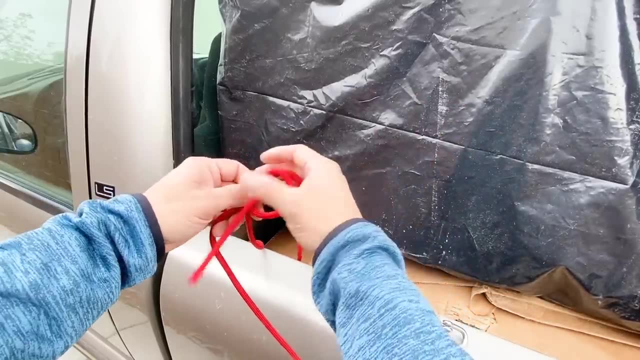 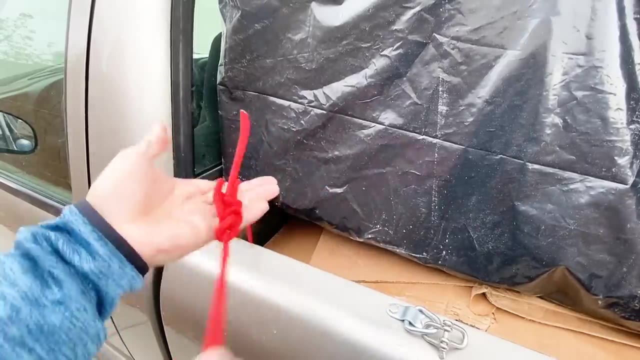 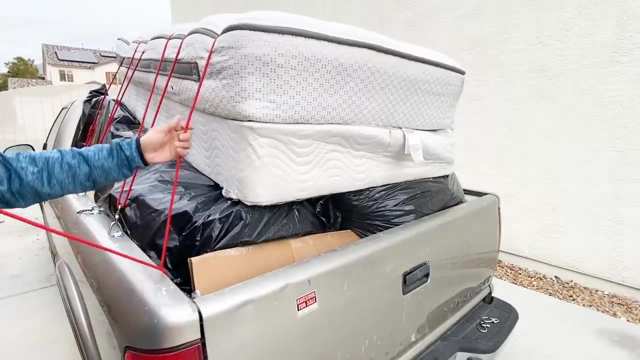 into my anchor point. i'll take the left side and pinch in my cow hitch. here we go. take this end, i'll thread it through, go around the standing portion and then thread it right back where i came from. pull everything tight. there we go. we're hooked into our last anchor point here. now i'm going to pull in a clove hitch. 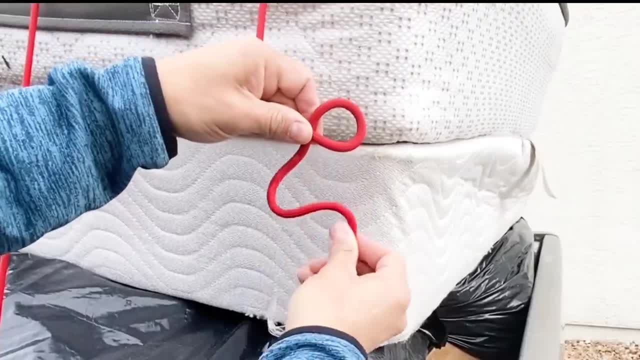 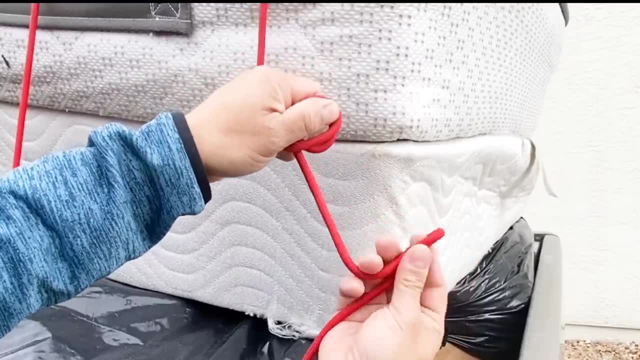 by twisting in a loop, i'll twist in another loop. there we go, and i'll lay them right on top of each other. i'm going to pull in a bite, then i'll thread this bite through my clove hitch. there we go. let's pull all that tight. 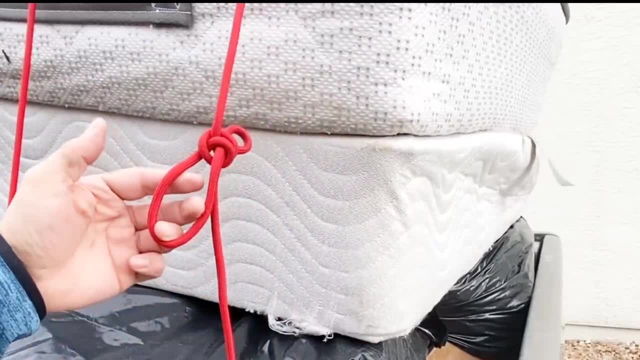 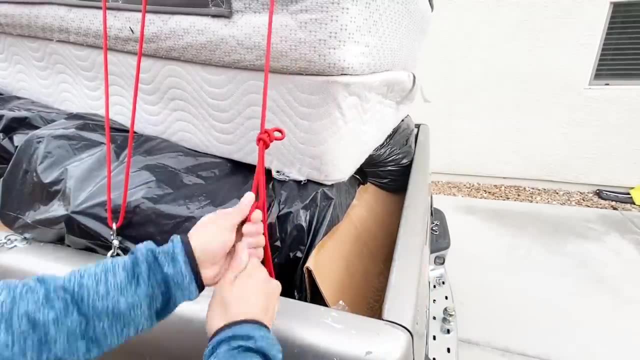 good. so now what i've done is given myself a loop where i can pull in some mechanical advantage. i'll take the end of my rope, thread it through and i'll pull everything tight. now i'll just use a couple half hitches to tie it off. 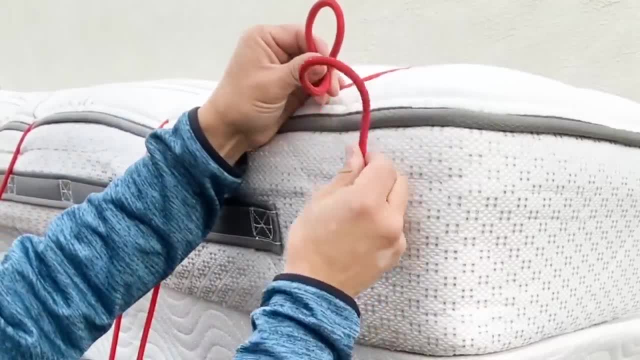 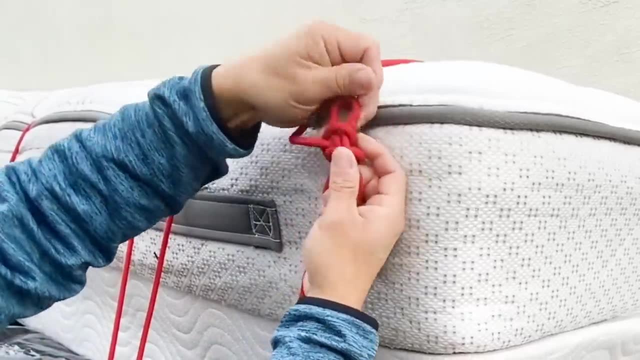 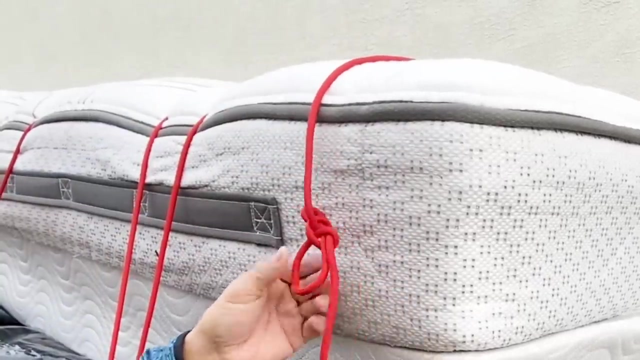 here it is one more time. twist in one loop, twist in another loop, right on top, grab a bite and i'll thread it through my clove. hitch there, tighten everything up. there we go, and now i have this bite here that i can run my cord through. 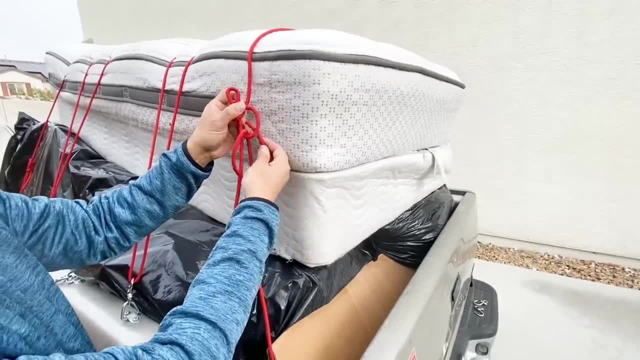 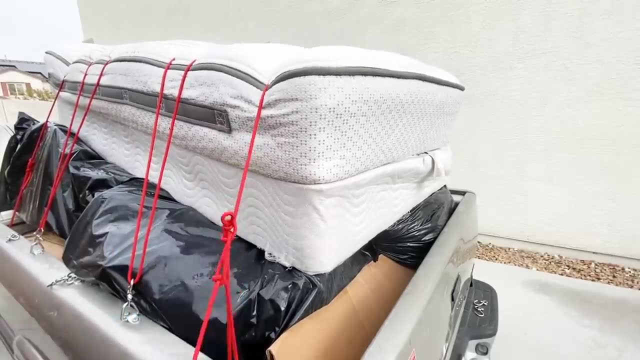 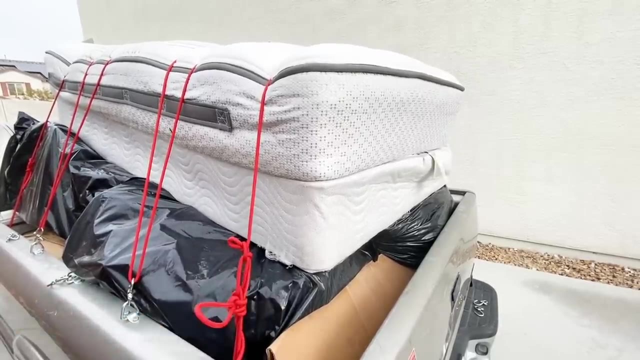 here's a little tip. i'll run it through once, go through one more time, and if i do it this way, it'll lock on itself and i don't have to hold it while i tie in my final half hitches. there we go, as you're learning the ropes. one great book is the ashley book of knots by clipper ashley. 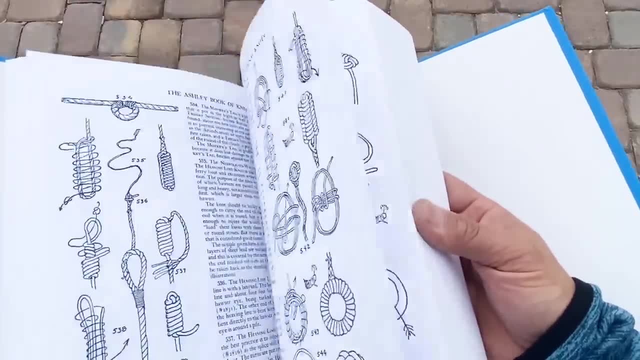 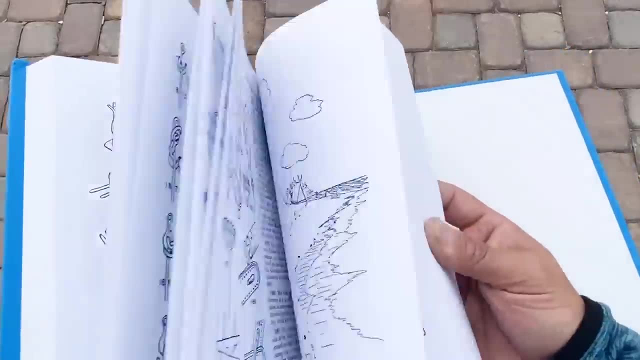 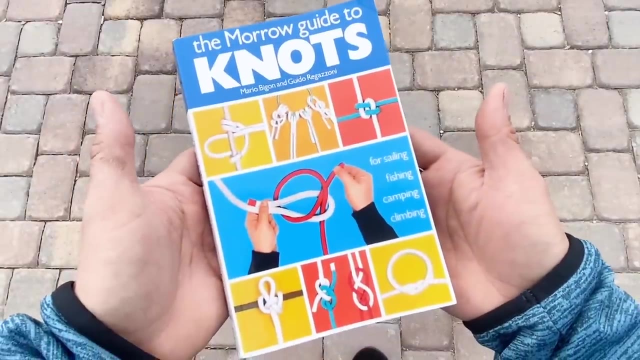 this book has thousands of knots in it now. it was written in 1947, so it wasn't out when nylon cord came out, but it still has plenty of knots for you to learn and explore, and there are other ways to learn about knots. another book i've enjoyed is the maro guide to knots. this one was written in 1982. 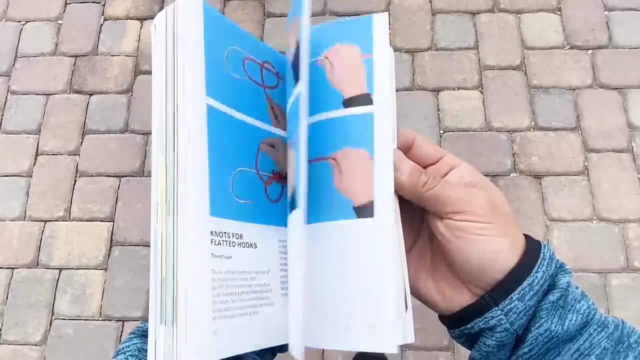 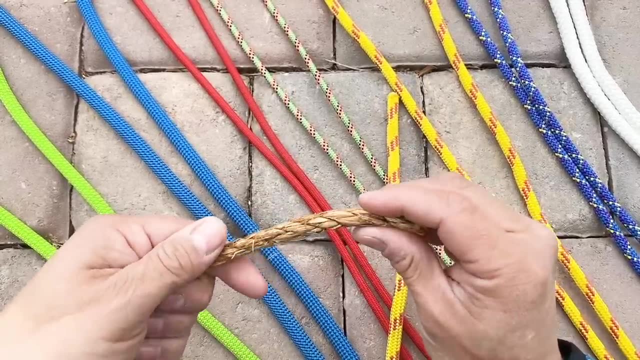 it has colored photos and there's plenty of knots in here for you to learn as well. let's take a second to talk about rope. there's two common styles you'll run across. one is twisted, where the rope is twisted together. the other is braided, and you can see that it is.